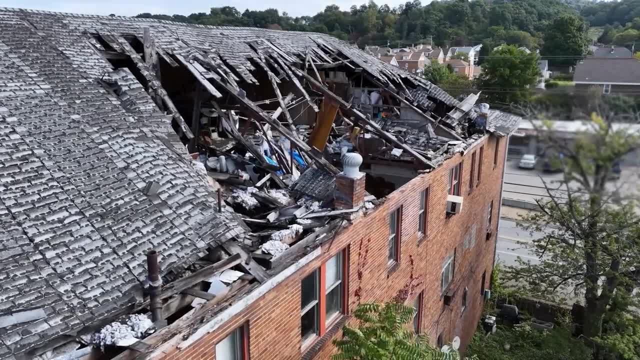 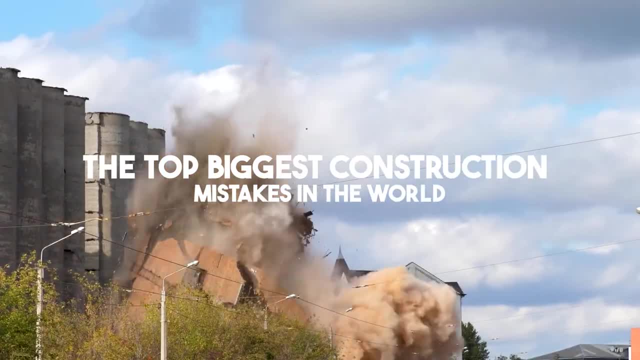 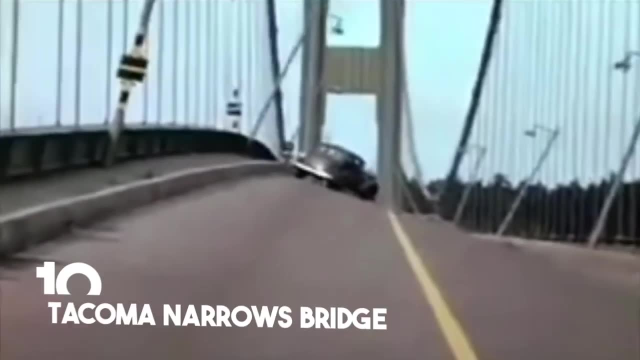 This is the height of construction disaster. Diving into the fascinating and hilarious world of construction calamities, Today we're tackling the big leagues, The top biggest construction mistakes in the world. Grab your hard hats and safety goggles because we're about to witness some epic engineering fails. Number 10. Tacoma Narrows Bridge. 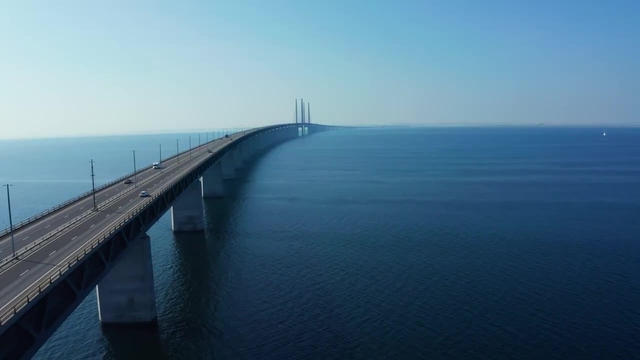 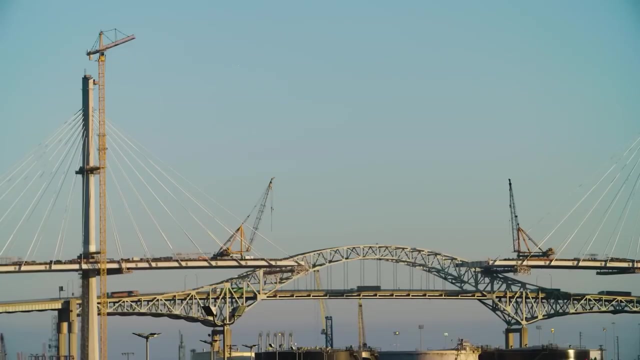 Imagine a bridge, majestic and modern, spanning a wide expanse of water. Now picture that bridge swaying wildly in the wind, cars clinging precariously to its undulating spine. That was the fate of the original Tacoma Narrows Bridge in Washington. 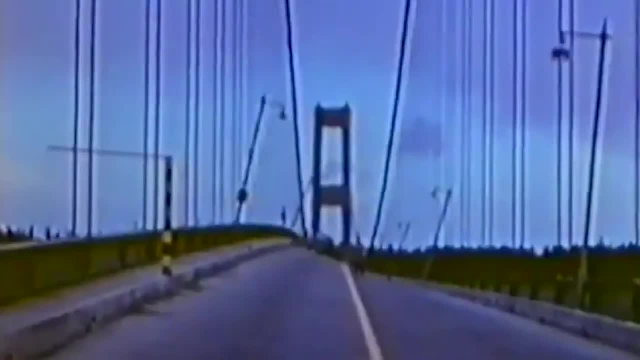 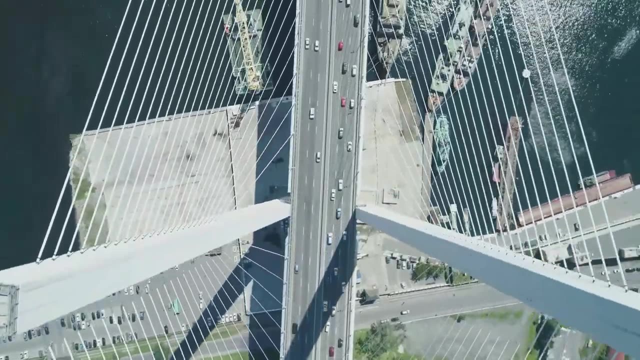 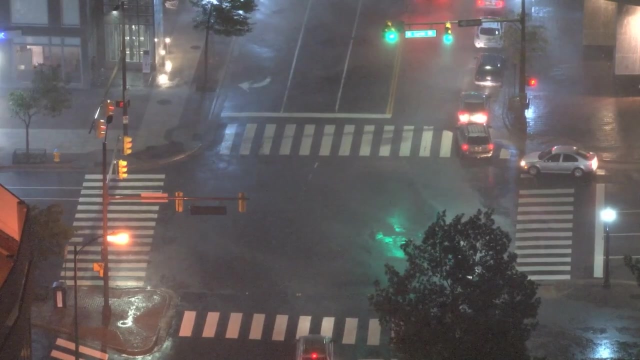 a colossal engineering marvel that unfortunately met its demise due to a fundamental oversight: Wind. Opened in 1940, the bridge was hailed as a technological marvel. Its sleek suspension design promised efficiency and grace. But what the engineers failed to take into account was the region's notorious wind gusts As soon as even a mild breeze hit. 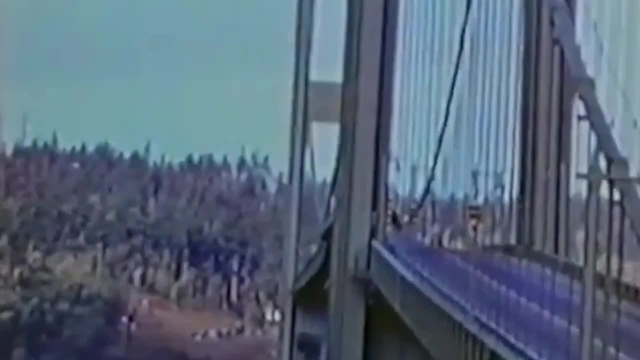 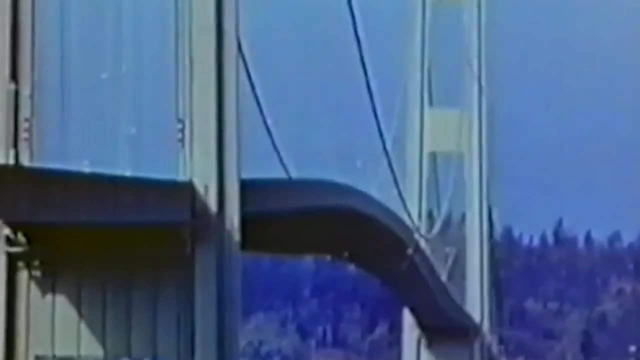 the bridge began to sway in an alarmingly rhythmic motion, earning it the nickname Tacoma. Galloping dirty Cars danced precariously, tires screeching in protest, as the steel ribbon writhed like a tormented serpent. The sight was both thrilling and terrifying. a spectacle of nature. 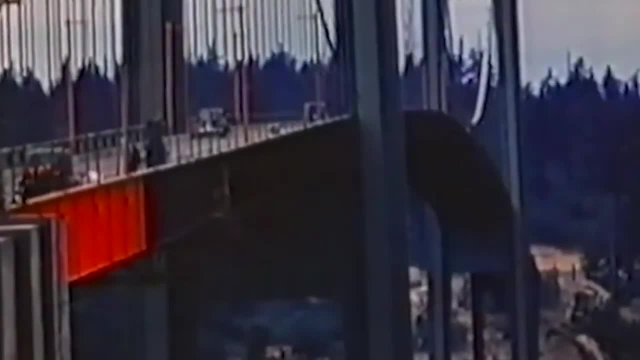 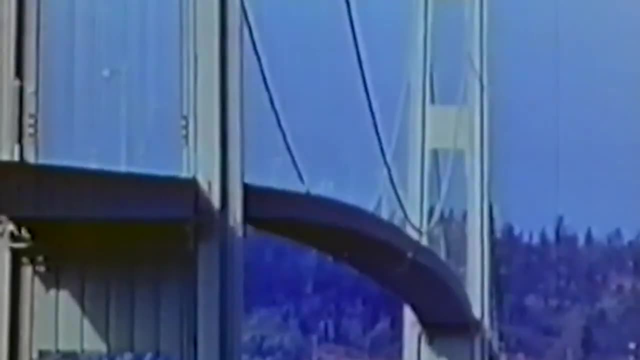 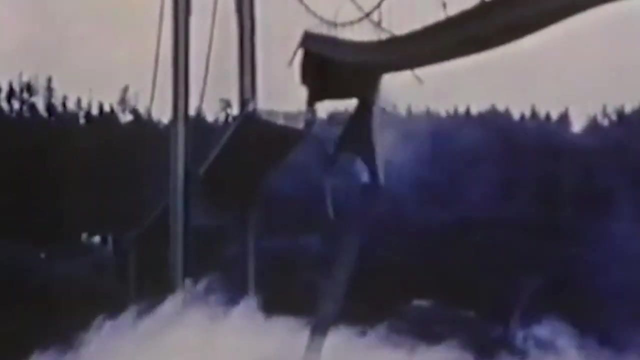 mocking human arrogance. This wasn't just an aesthetic issue. The vibrations threatened the bridge's structural integrity Just four months after its grand opening, under the watchful eyes of thousands of horrified spectators, dirty, buckled and snapped Cars plunged into the icy waters below. 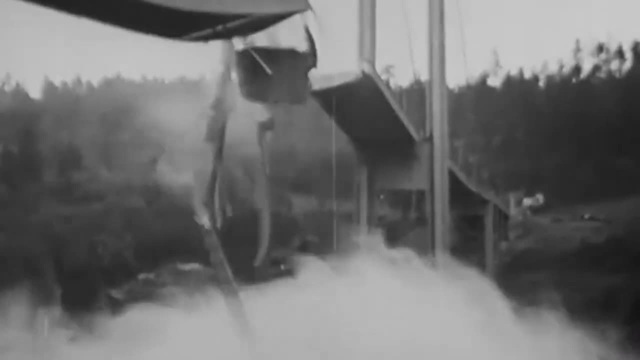 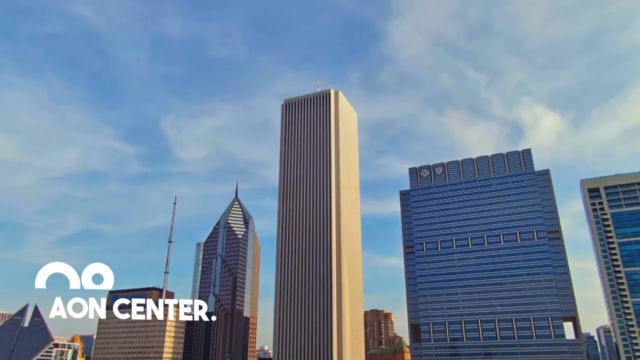 thankfully with no loss of life. The collapse was a brutal wake-up call, forever etching the importance of wind testing into the annals of engineering history, Number 9. On Center. Chicago's On Center, once envisioned as a beacon of progress, earned a rather less. 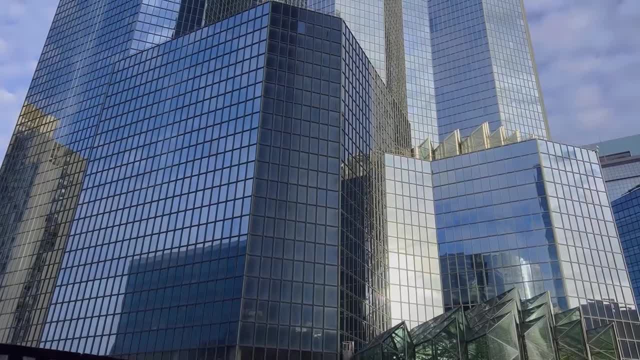 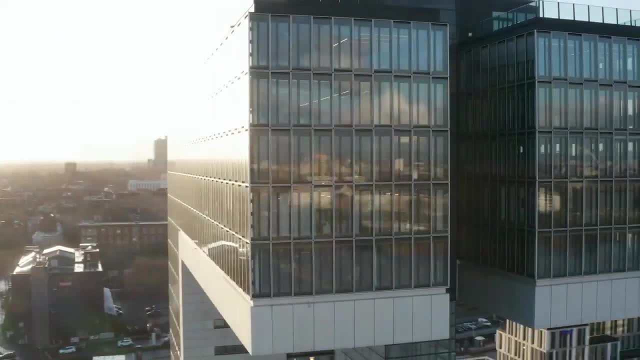 flattering nickname: the Sunburn Skyscraper. This sleek glass-clad behemoth had a serious case of architectural agoraphobia, reflecting the sun's rays with laser-like intensity. The result: Cars parked nearby spontaneously combusted, their paint blistering under the concentrated heat. 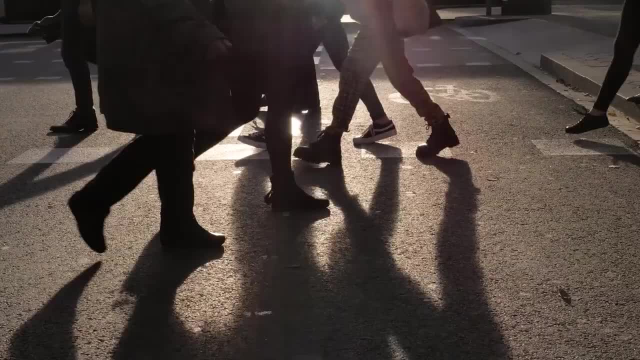 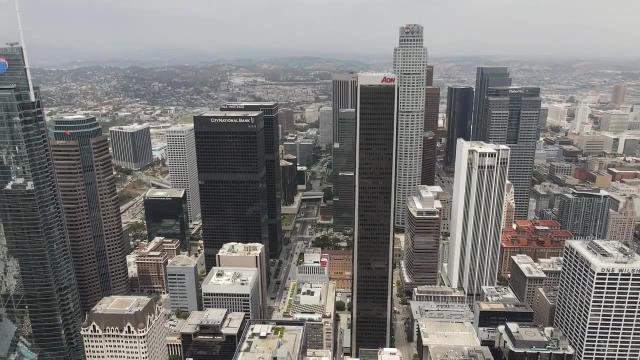 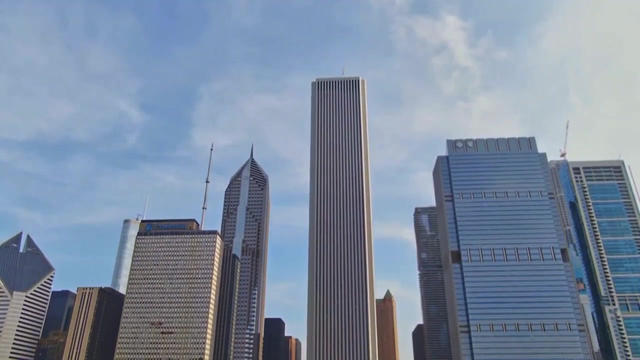 Pedestrians became involuntary toast, stepping gingerly around patches of sidewalk, sizzling at 130 degrees Fahrenheit. The culprit The On Center's concave glass façade designed to mimic a giant bean. This curvature acted like a magnifying lens, focusing the sun's rays into 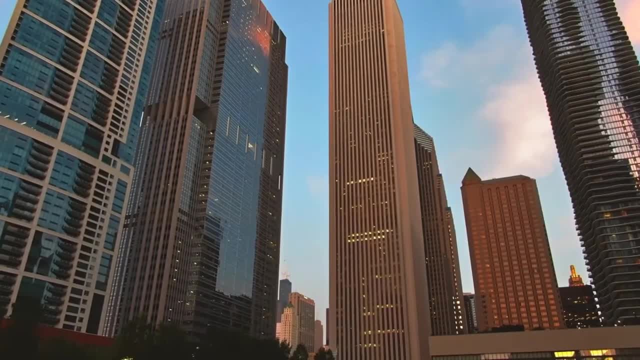 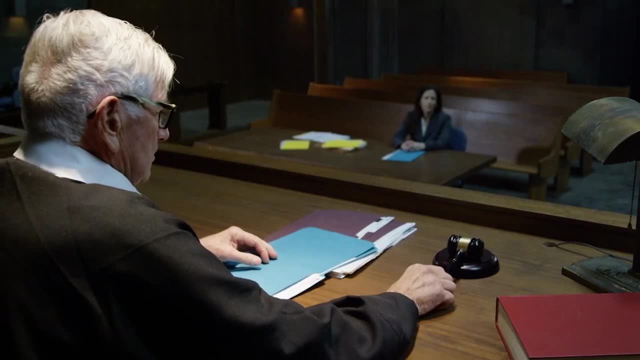 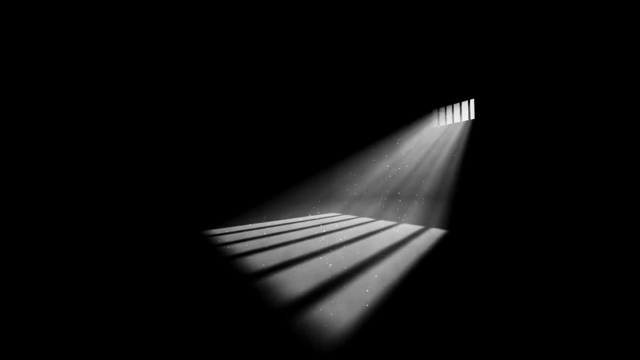 localized beams of fiery fury. The unintended consequences were both comical and potentially potentially tragic. imagine spontaneous hair combustion. After a barrage of lawsuits and singed eyebrows, the architects devised a solution. Giant metal fins were added to the building, casting awkward shadows and transforming the once sleek bean. 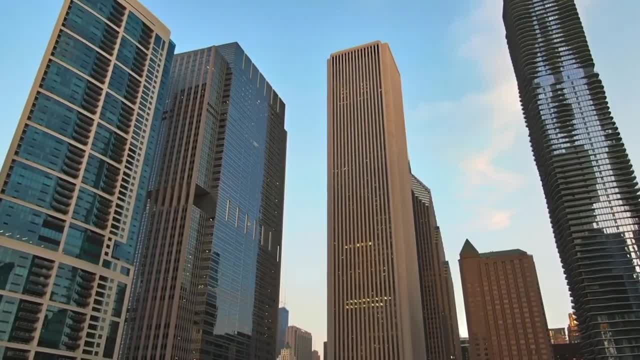 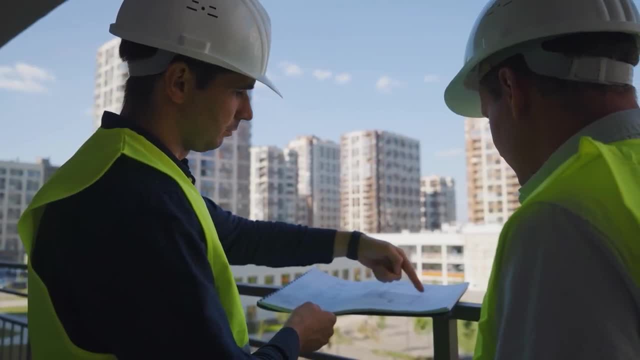 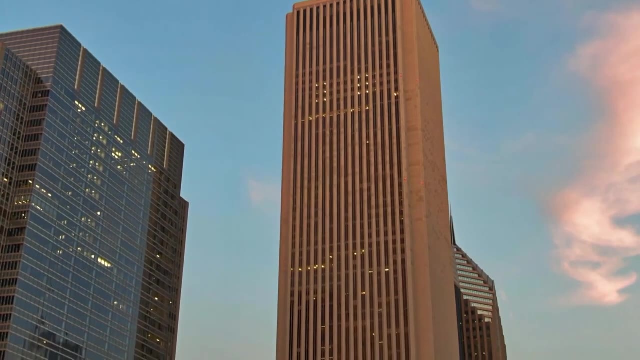 into a somewhat prickly mutant. The On Center stands as a monument to the unintended consequences of architectural hubris. It's a cautionary tale about the importance of considering practicalities alongside aesthetics, a reminder that shiny things can sometimes burn the very things they're supposed to impress. 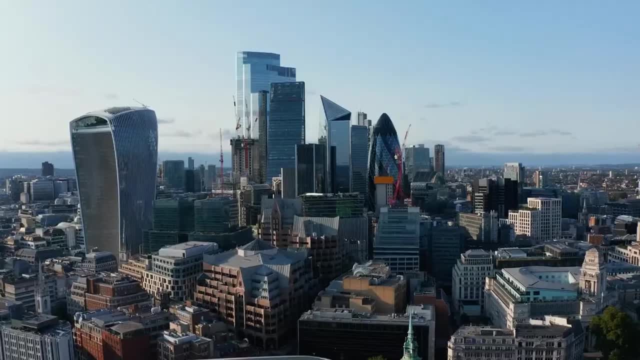 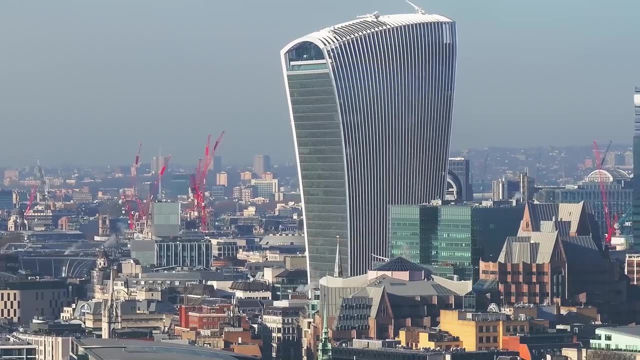 Number 8. Walkie-Talkie Across the pond. London's Walkie-Talkie faced a different, albeit equally perplexing, problem. This futuristic edifice with its bulging glass facade wasn't melting cars or scorching pedestrians. 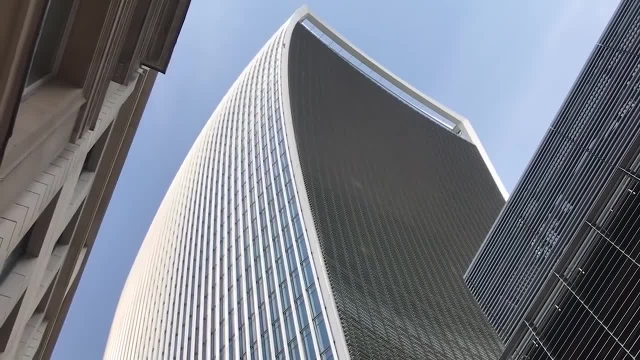 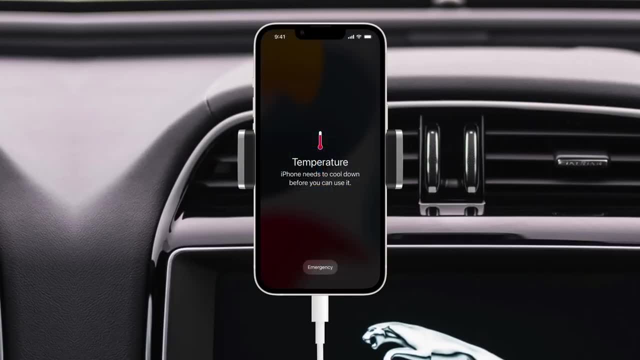 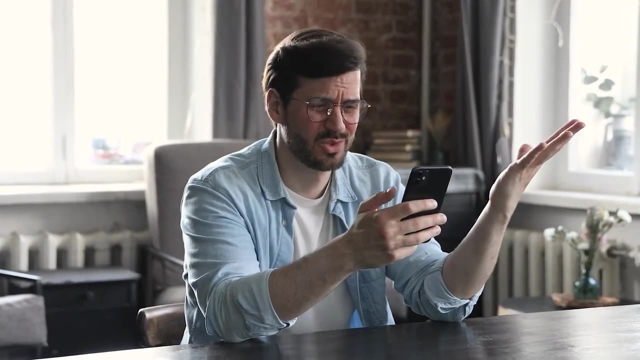 No, it was frying their phones. The curved glass acted like a giant parabolic dish, focusing radio waves into concentrated blasts that could not be seen. Imagine the scene: Businessmen glued to their Blackberries suddenly plunged into a digital abyss: Emails, froze, calls dropped. social media became a desolate wasteland. 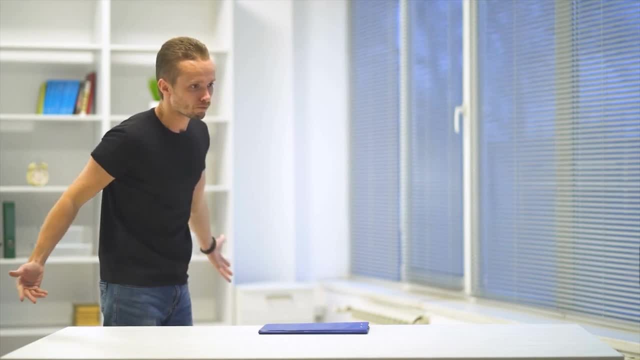 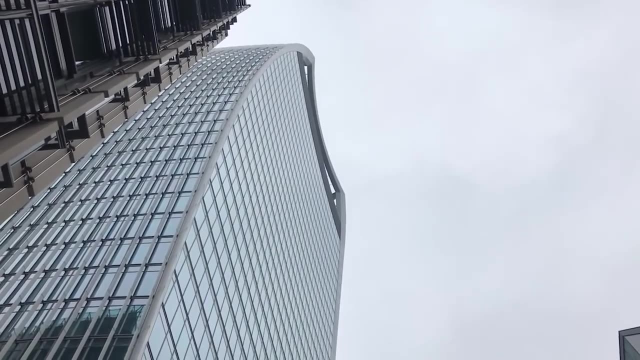 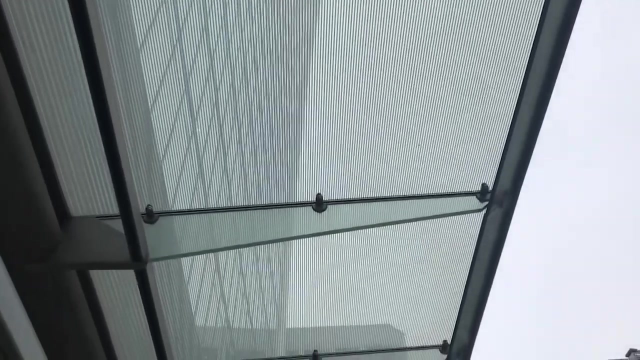 The frustration was palpable, The productivity non-existent. The culprit, Again, the building's unique design. The reflective glass concentrated radio waves like a microwave oven, turning the surrounding area into a mobile communication dead zone. The solution: Installing giant mesh screens around the building, essentially turning 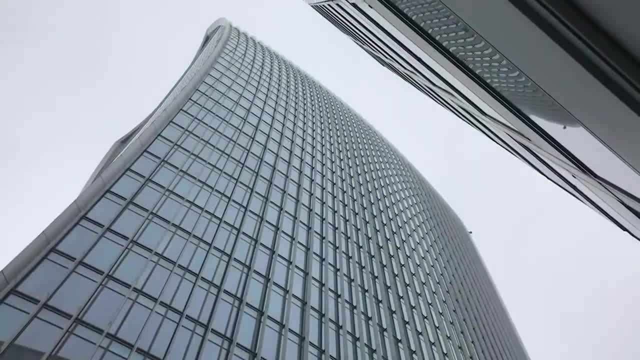 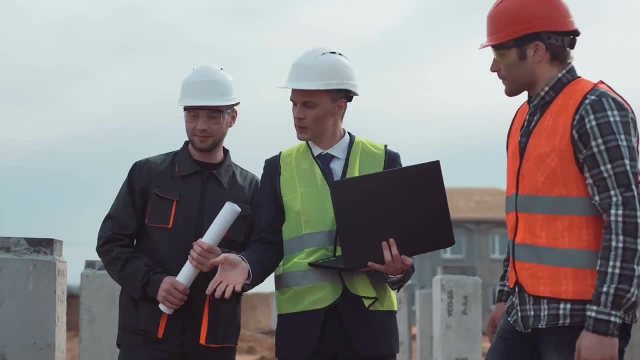 the once-sleek Walkie-Talkie into a slightly bug-eyed alien visitor. The foam-frying fiasco became a global punchline, highlighting the unforeseen challenges that can arise when pushing the boundaries of architectural design. Number 7. Millennium Bridge. 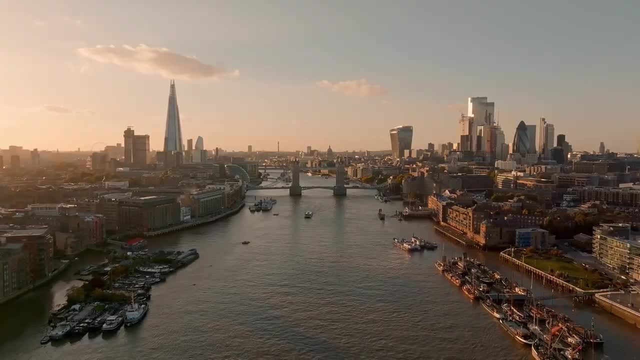 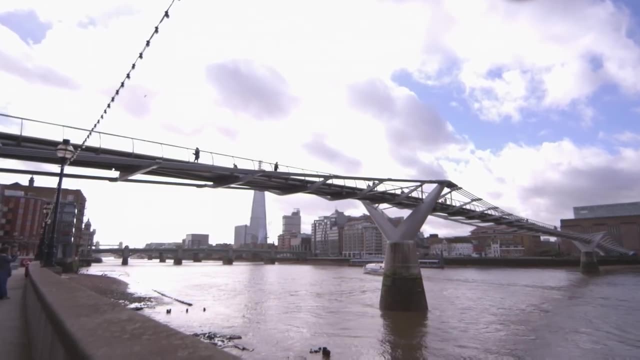 The Millennium Bridge, London's futuristic pedestrian bridge spanning the River Thames, promised to be a symbol of the city's forward-thinking spirit. But on opening day in 2000,, the Millennium Bridge, London's futuristic pedestrian bridge which was built in the early 2000s, took a nose-dive, quite literally. 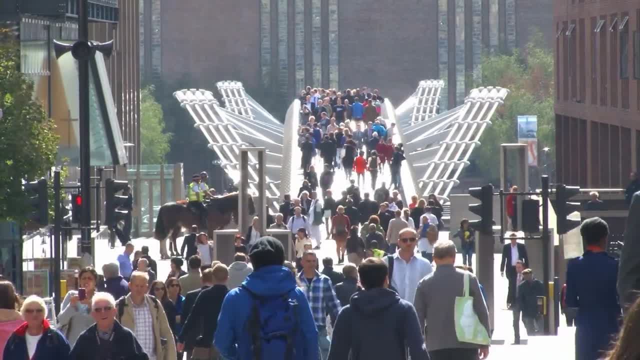 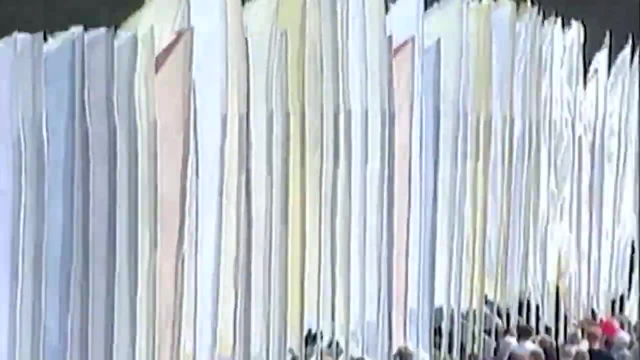 As hundreds of eager Londoners stepped onto the bridge, a strange phenomenon occurred. The sleek, suspended walkway began to sway rhythmically, a motion imperceptible at first, then slowly amplifying into a disconcerting shimmy. Within minutes, the bridge was undulating. 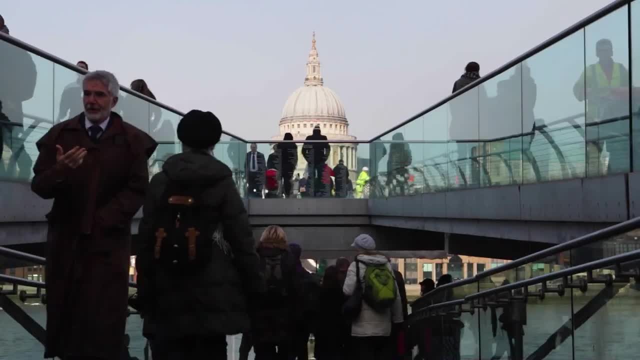 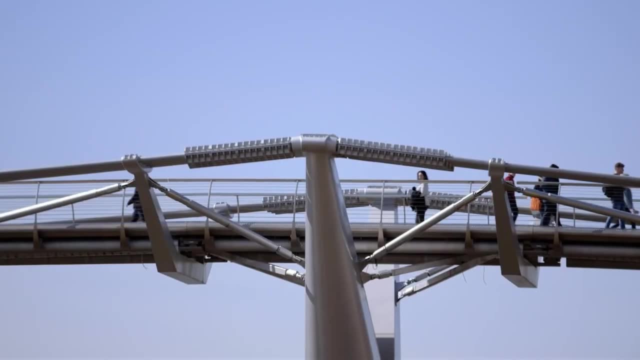 like a giant trampoline. alarms were blaring and pandemonium ensued. The culprit: A miscalculation in pedestrian dynamics. Engineers absorbed on the bridge's structural integrity and hadn't considered how the rhythmic footsteps of a large crowd 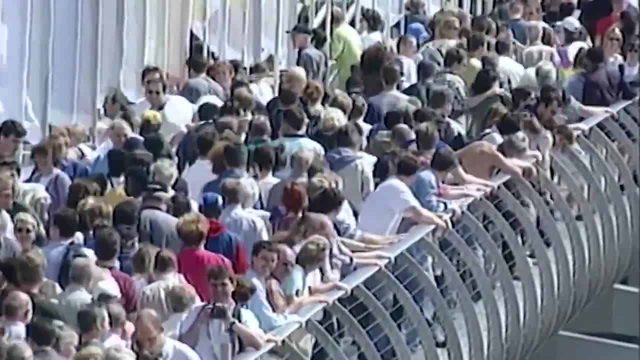 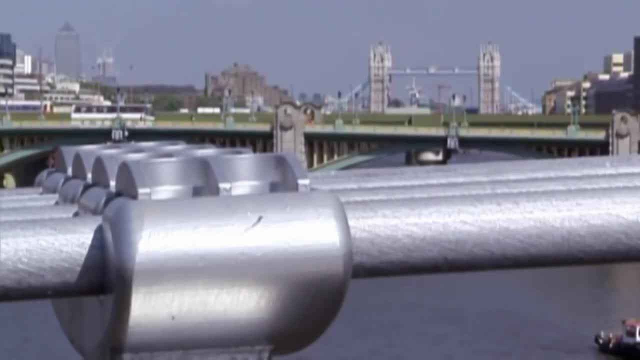 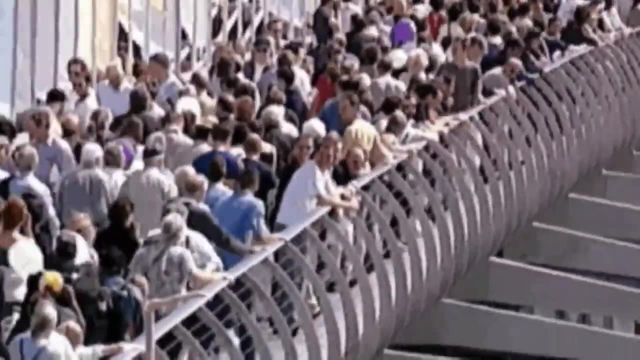 would synchronize with the bridge's natural frequency, setting it rocking like a child's playground seesaw. This lateral sway, exacerbated by the bridge's lightweight design, sent shivers not just through the structure, but also through the confidence of the city. The wobbly bridge incident, which was quickly labeled, caused humiliation throughout the 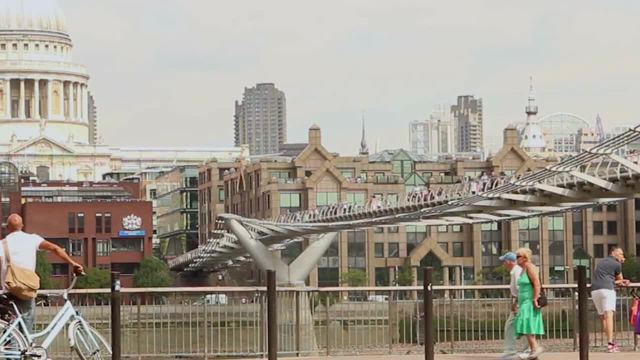 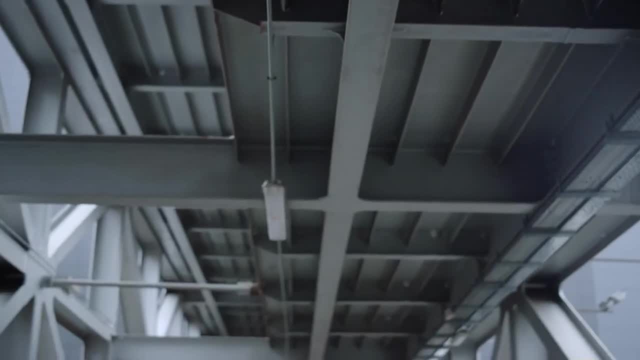 world Without delay. the bridge was closed for two years and had to undergo an embarrassing retrofitting procedure. The bridge was closed for two years and had to undergo an embarrassing retrofitting procedure. To combat the swinging motion, engineers built cumbersome hydraulic pistons and enormous 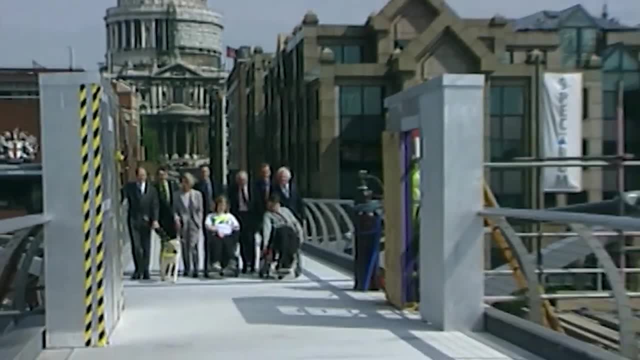 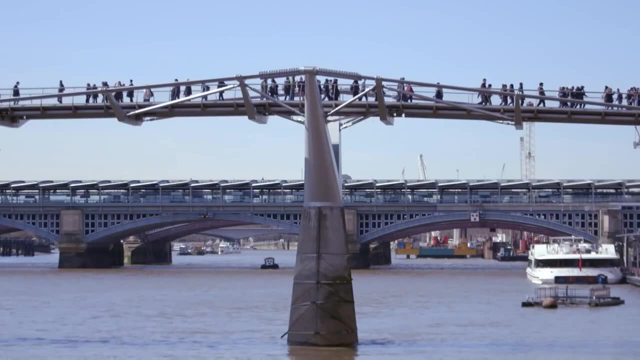 dampers beneath the deck. Even while they worked well, these dampers were not at all the elegant, undetectable solution one would anticipate from a project of this caliber. Reopened in 2002,, the bridge was eternally altered by its unsteady beginnings. a lesson: 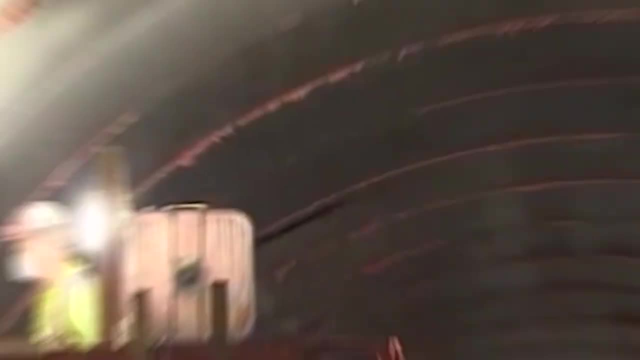 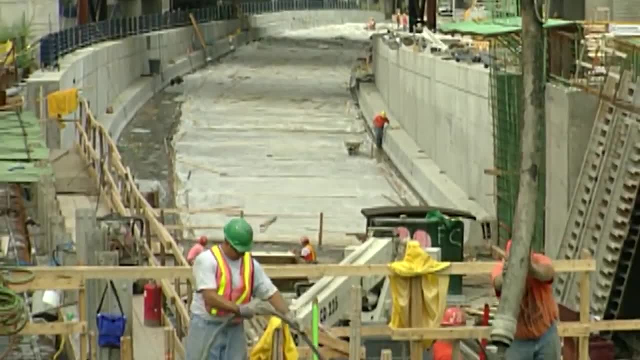 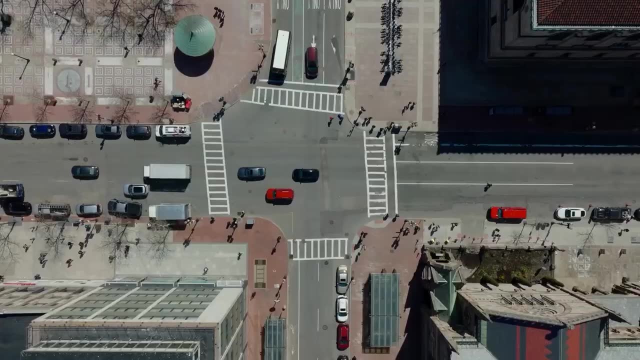 This project is so ambitious and complex that its very name conjures images of subterranean nightmares and budgetary black holes. Conceived in the 1960s to bury Boston's choked-up highway system, the Big Dig promised a traffic-free utopia. What it delivered was a decade-long. 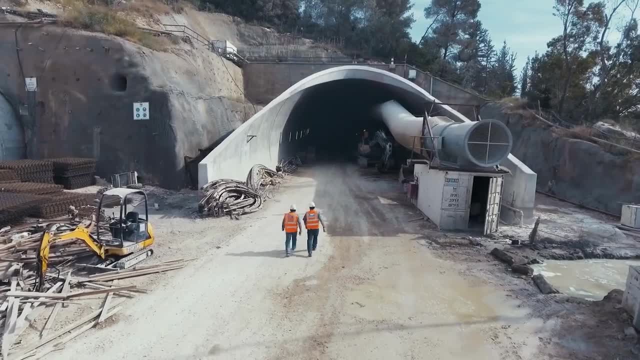 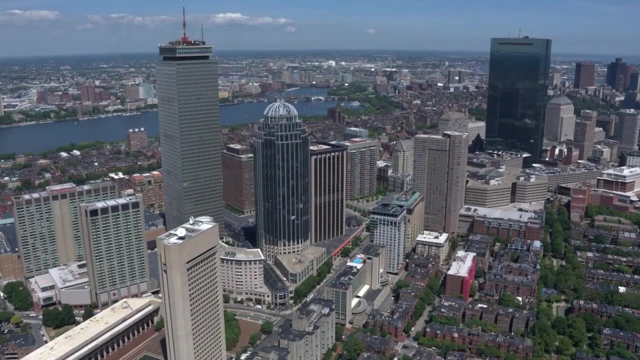 labyrinth of construction, a symphony of jackhammers and detours and a fiscal hangover of epic proportions. The challenges were monumental: Burrowing beneath a historic city, excavating mountains of earth and navigating a mountainous landscape. the Big Dig was inspired by the enigmatic 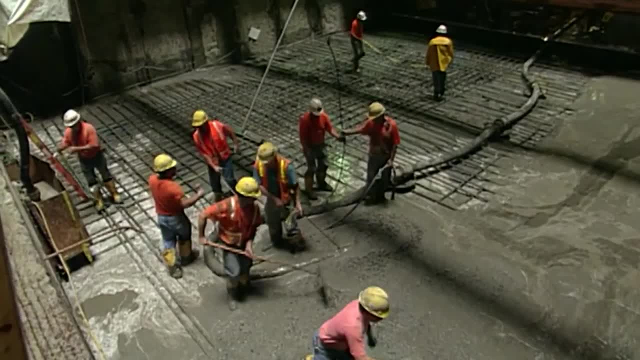 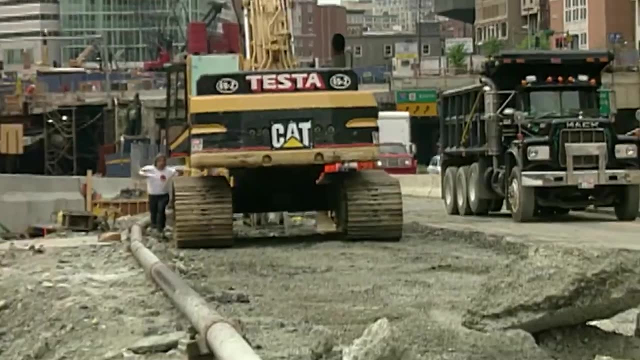 maze of utilities, each day seemed to unearth a new obstacle. Leaks sprung like unwanted geysers, flooding tunnels and strolling traffic. Cost overruns became as routine as potholes, ballooning the initial $5 billion estimate to a staggering $22 billion. 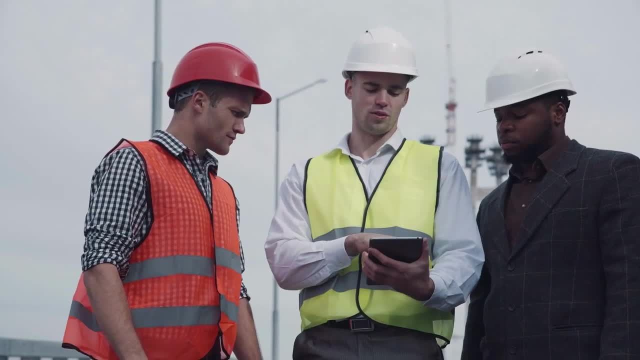 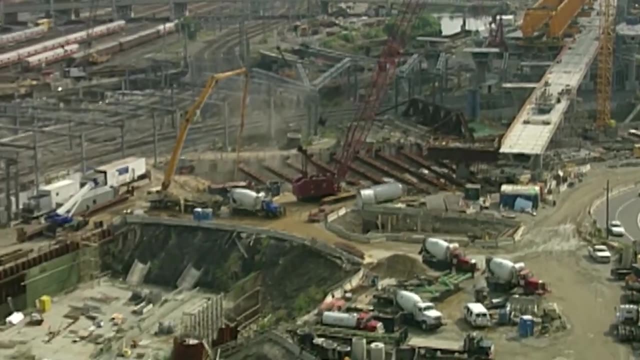 The project, originally slated for a decade, crawled into its 16th year, leaving Bostonians weary and wondering if they'd ever see daylight again. But beyond the logistical nightmares, the big dig had a darker side. Construction sites became havens for corruption, with kickbacks and scandals. 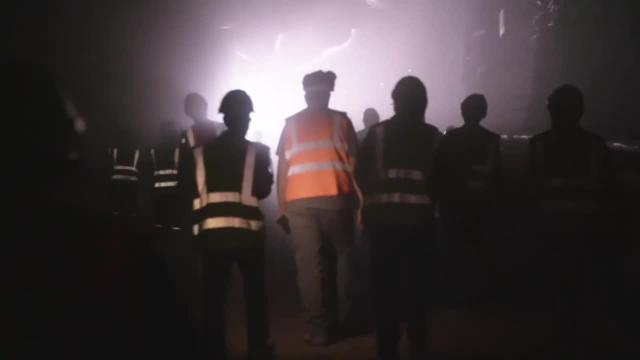 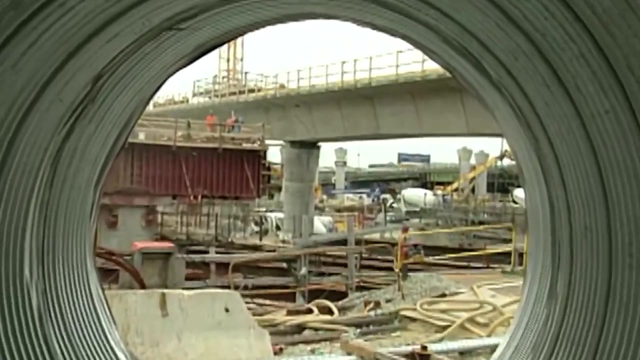 swirling like dust clouds. Worker safety was another issue, with several fatalities casting a grim shadow over the project. At last, the dust settled to some extent in 2007.. Though it still had the marks from its difficult beginning, the big dig was deemed finished. 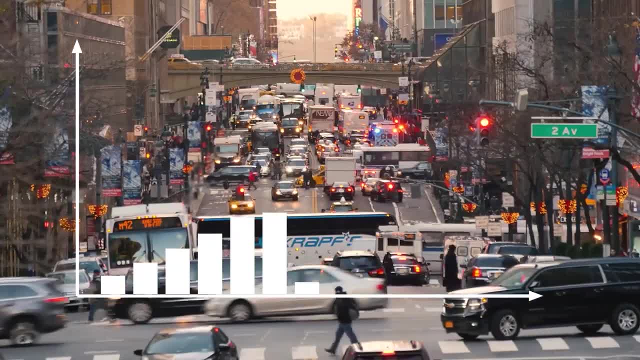 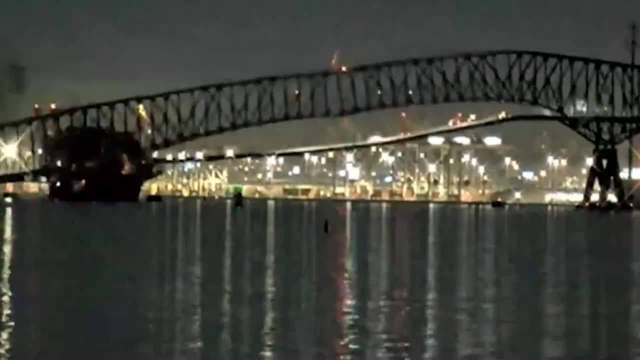 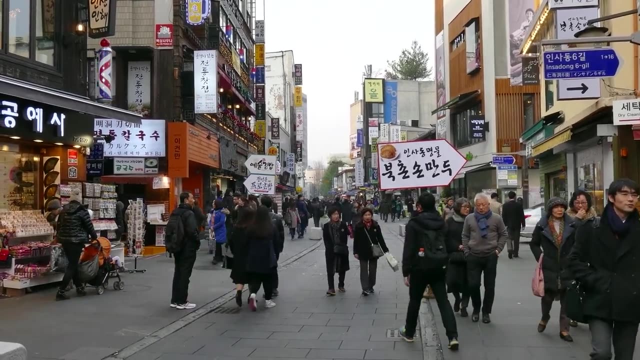 Although it helped ease some traffic congestion, the actual financial and human cost serves as a warning about the dangers of unbridled ambition and the drawbacks of large-scale undertakings. Number 5. The Seongsu Bridge Collapse In 1994, a tragedy unfolded in Seoul, South Korea, leaving behind a gaping wound in the 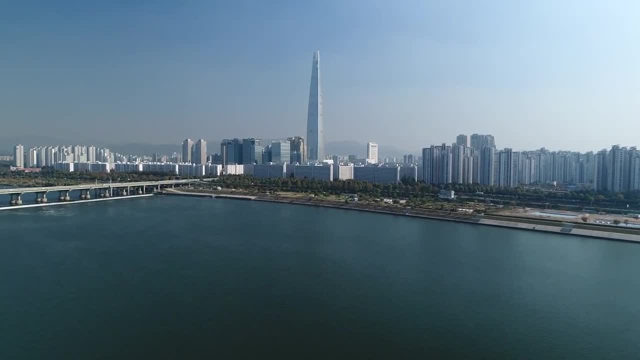 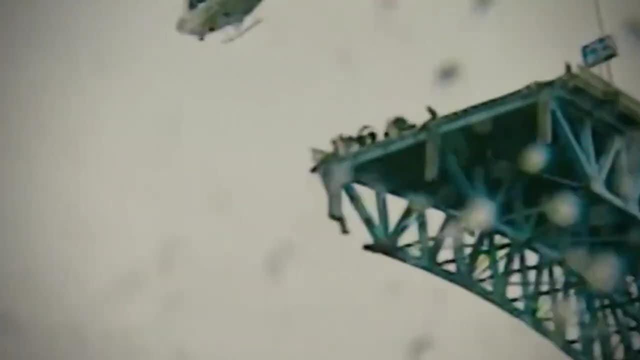 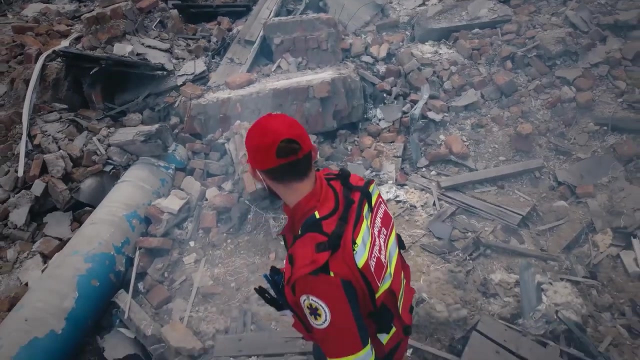 city's skyline and a deep scar on the national psyche. The Seongsu Bridge, then under construction, spectacularly collapsed, sending tons of twisted steel and concrete plummeting onto the unsuspecting street below. The toll was horrific: Thirty-two workers perished, were crushed and were buried. 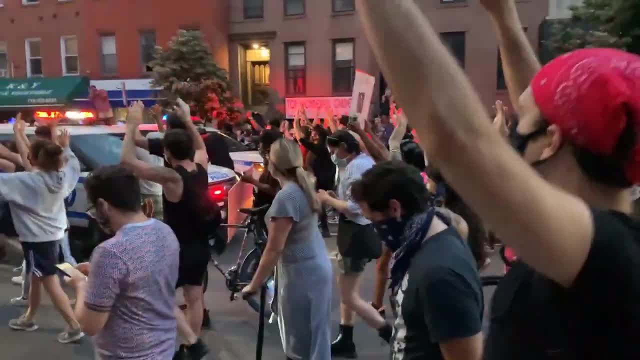 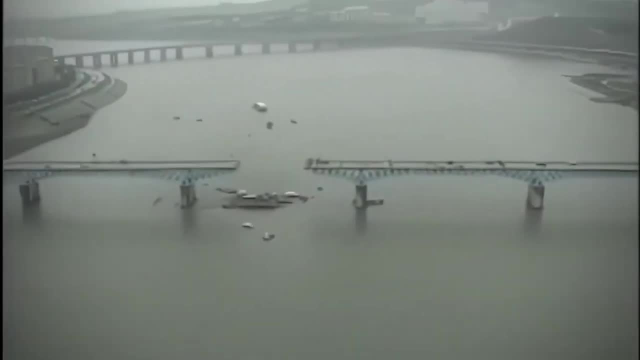 in the city. The bridge was built in the 19th century. The bridge was built in the 19th century. The initial shock gave way to anger and accusations. Investigations revealed a fatal design flaw in the bridge's support beams, a critical error that, if caught, could have. 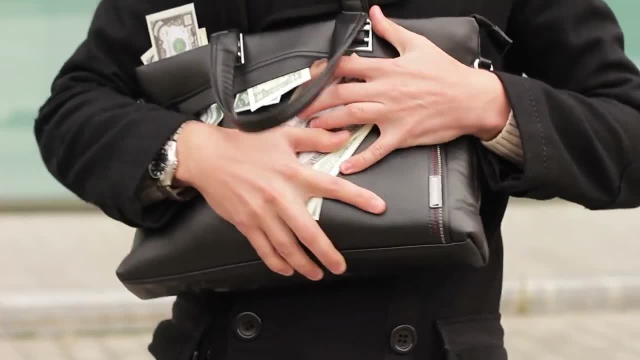 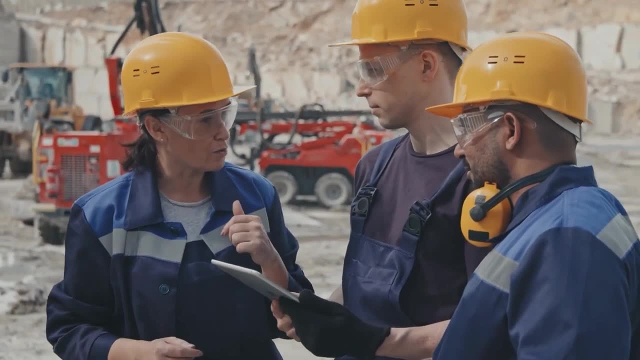 prevented the entire disaster. Greed and corruption further tainted the picture, with reports of shoddy materials and lax safety standards, contributing to the bridge's untimely demise. The fall of the Seongsu Bridge serves as a sobering reminder of the results of carelessness. 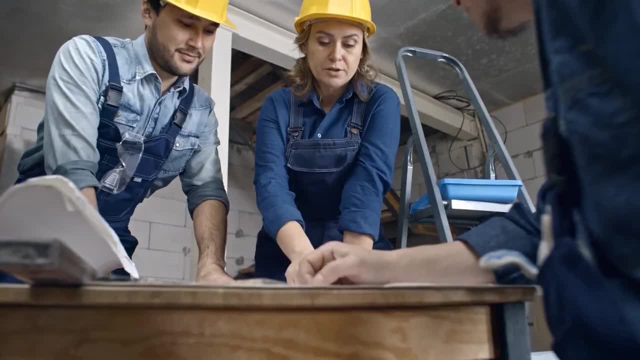 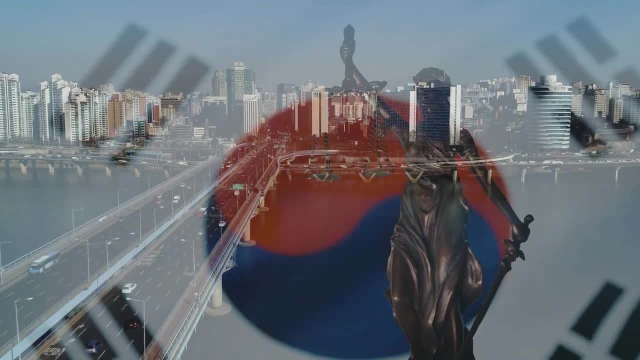 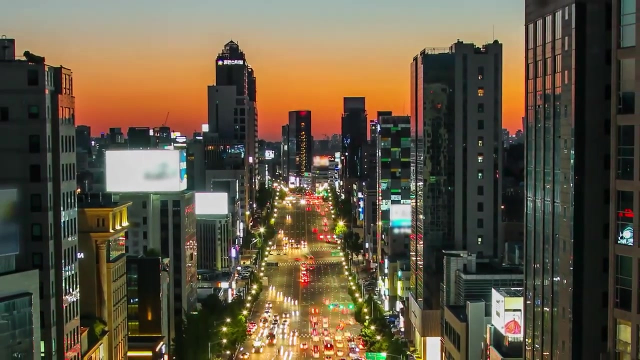 and misguided objectives In the construction sector. it serves as a sobering reminder to put safety and human life before expediency and profit. Following the incident, South Korea pledged to never allow a disaster of this magnitude to happen again and implemented extensive changes to its building procedures. 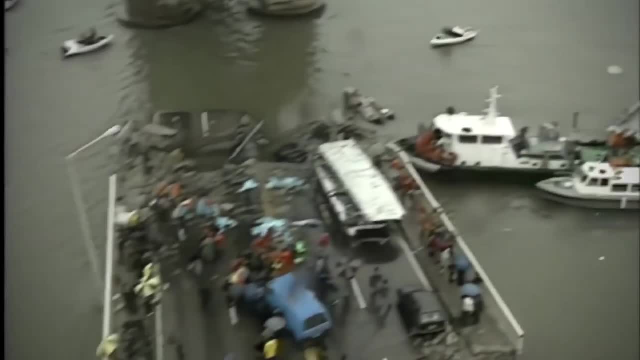 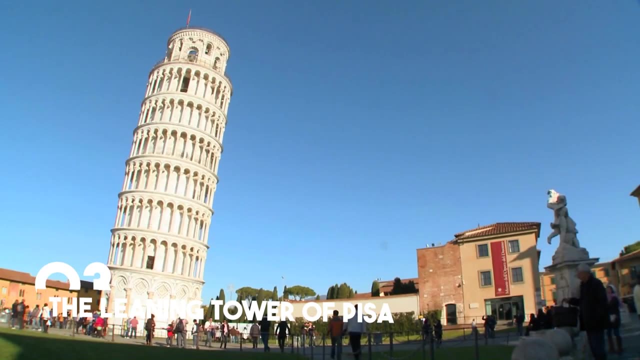 The Seongsu Bridge is still a somber reminder of the human cost of engineering errors and the responsibility that comes with using one's creative ability. Number 3. The Leaning Tower of Pisa. The Leaning Tower of Pisa may be a tourist magnet, but it began as a colossal engineering. 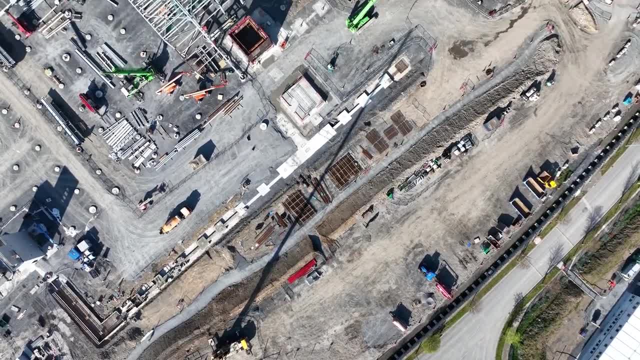 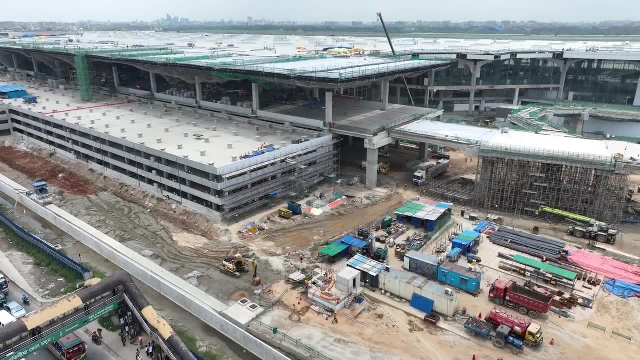 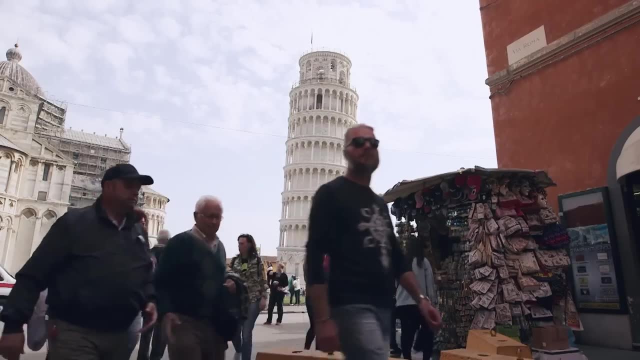 blunder. Built on unstable marshy soil, the foundation was a mere three meters deep, woefully inadequate for the ambitious eight-story plan. Construction began in 1173, but before reaching the third floor the tower started its iconic lean Panicked. engineers tried to compensate by building higher columns on the tilting side. 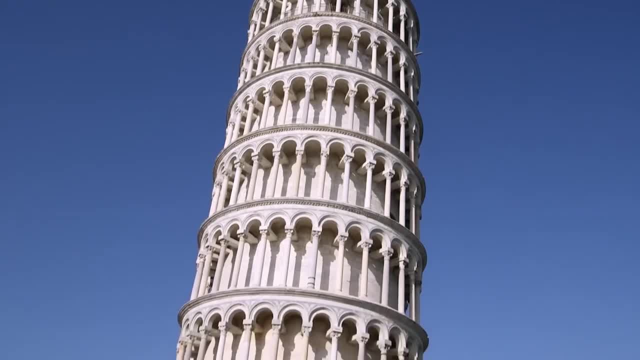 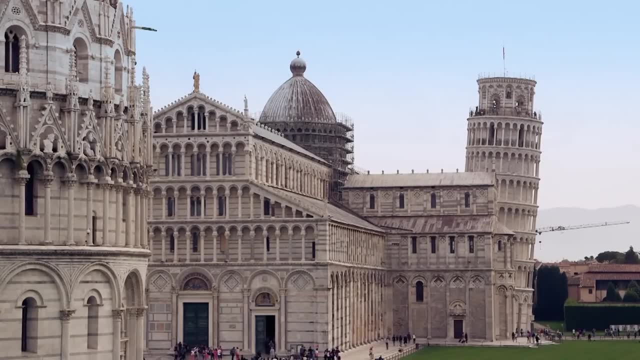 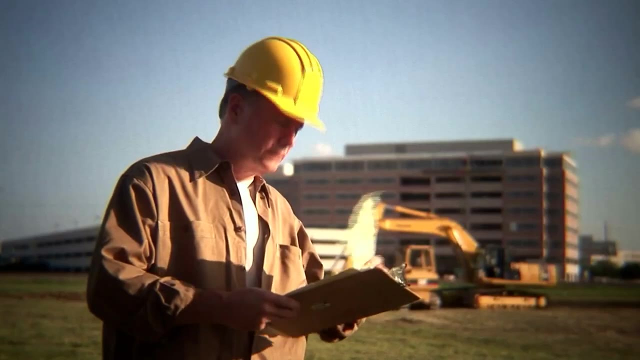 but it simply exacerbated the problem. The Leaning Tower became a leaning tower of cards, defying gravity. with every inch it tilted. Despite several stable verticalization efforts over the centuries, its tilt continued to increase, reaching a precarious 5.5 degrees by the 1990s. Closure loomed. Engineers devised a daring plan: extracting 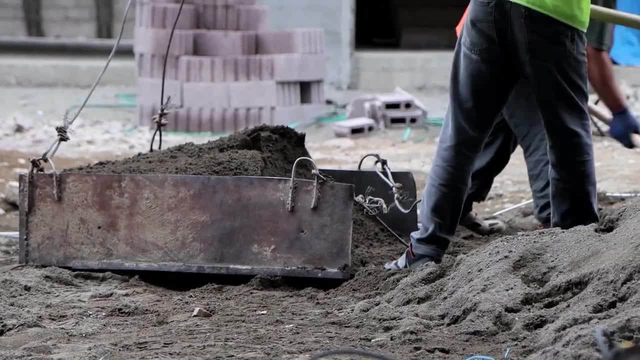 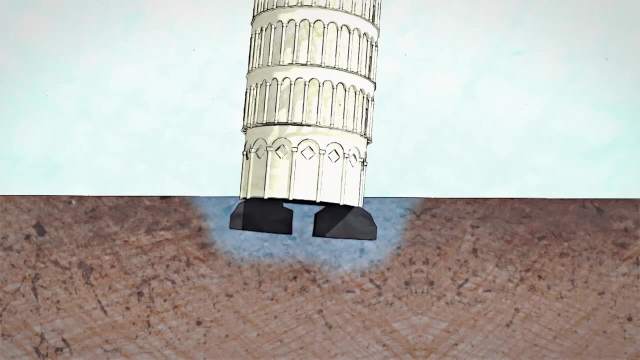 soil from beneath the leaning side to slowly nudge it back upright. It was a gamble, but successful. By 2001, the tower had miraculously straightened by 45 centimeters, the first time it had leaned less in centuries. The Leaning Tower stands as a monument not just to 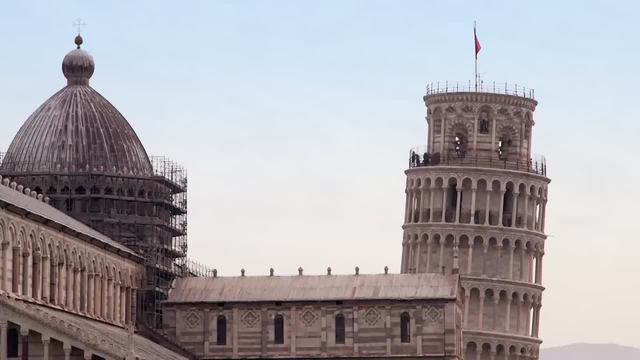 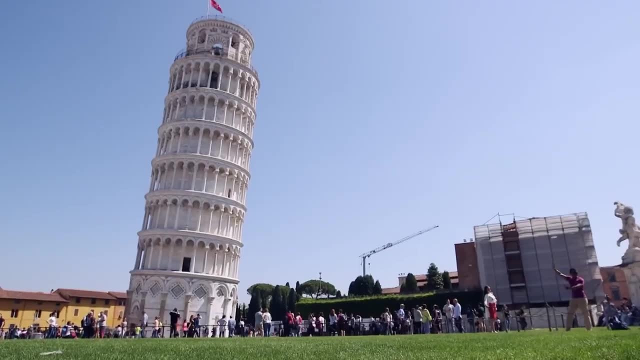 architectural beauty, but also to the folly of miscalculating gravity and the ingenuity it takes to recover from mistakes. It's a tilted testament to the enduring power of human ambition. A tourist magnet built on a foundation of error, forever teetering between triumph and catastrophe. 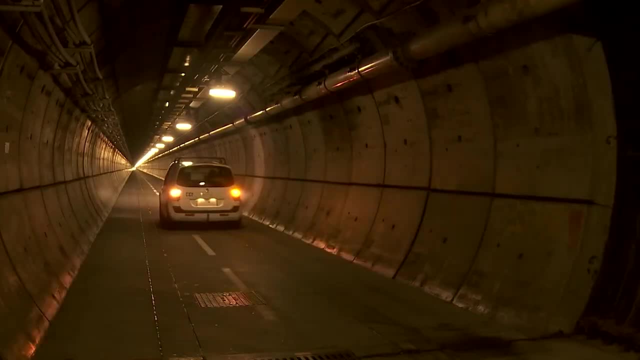 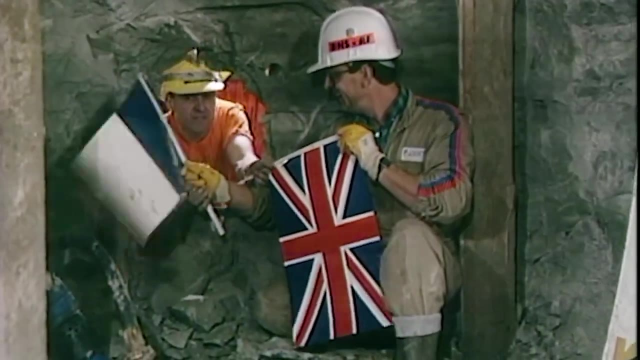 Number 2. The Channel Tunnel. The Channel Tunnel, ambitiously dubbed Le Tunnel sous la Manche, meaning the tunnel underneath the channel, aimed to revolutionize travel between England and France. It promised a speedy train ride beneath the Leaning Tower, and it was a success. The Leaning Tower was a. 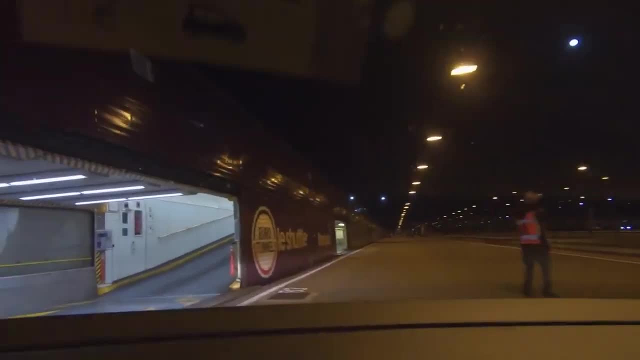 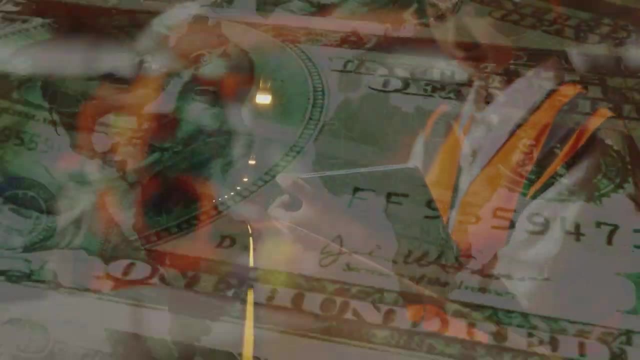 great example of this. It was the first tunnel in the history of the Leaning Tower to be able to rotate the English Channel, whisking passengers and vehicles from Folkestone to Calais in just 35 minutes. Yet instead of becoming a beacon of European unity, the project became synonymous. 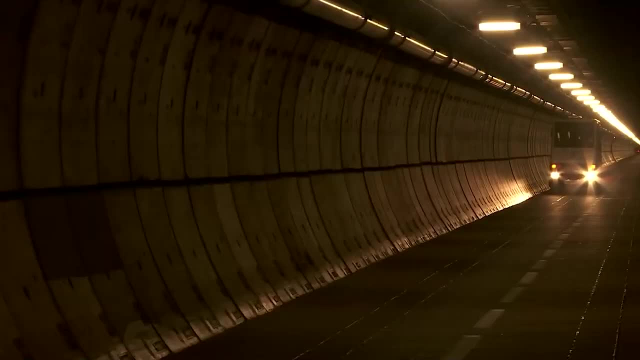 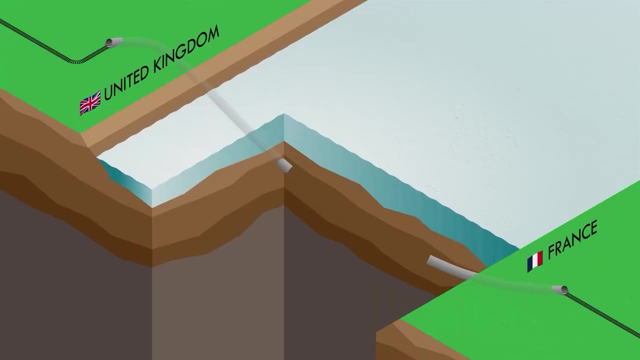 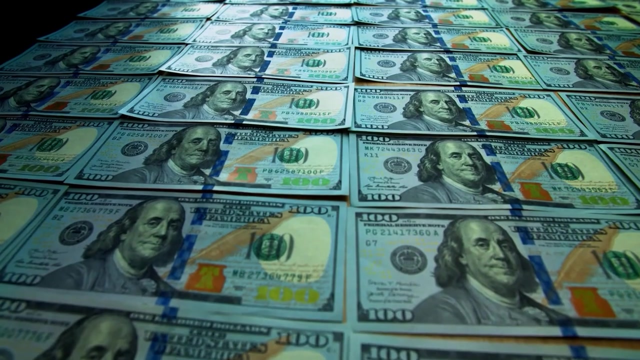 with engineering headaches and financial woes. Born in the 1980s and officially opened in 1994, the Channel Tunnel was a behemoth. Spanning 50 kilometers, it boasted the longest underwater section of any tunnel in the world, burrowing 75 meters below the seabed. This engineering marvel, 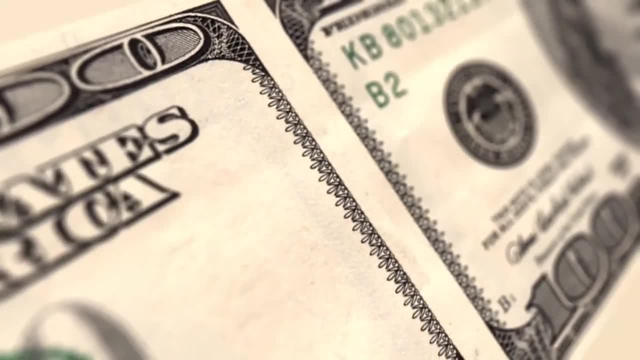 was the first tunnel in the world to have been built since the early 1980s and it was a huge feature of the Channel Tunnel in the history of the Leaning Tower. The Channel Tunnel was the largest ever built in the world, with an area of 100,000 square. 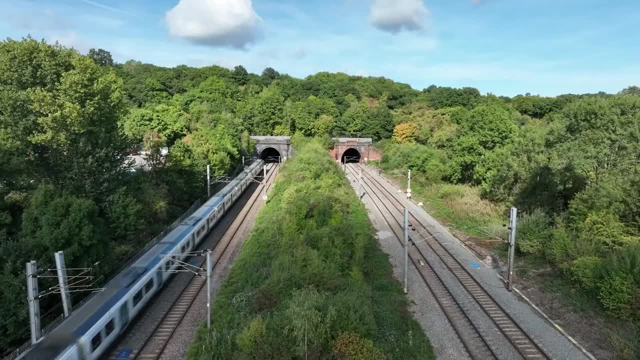 feet, with a total area of 7.4 million square meters, A staggering 12 billion pounds- around 15 billion dollars at the time- making it the largest privately funded construction project in history. However, trouble started brewing even before the first train departed. Technical difficulties plagued the construction, including fires that nearly halted the project altogether. Cost overruns mounted, ballooning by nearly 80 percent above the initial estimate. Public skepticism turned into ridicule with the project derisively nicknamed the Failed Tunnel. Still, persistence won out in the midst of the mayhem. 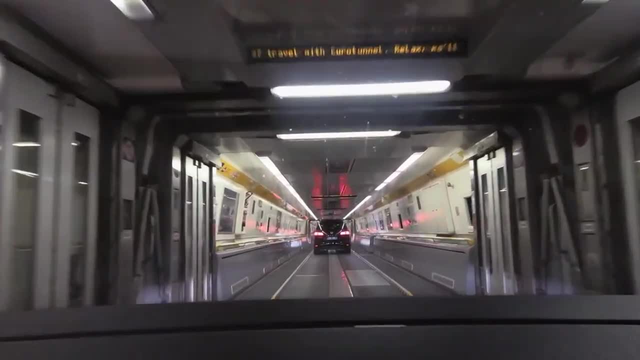 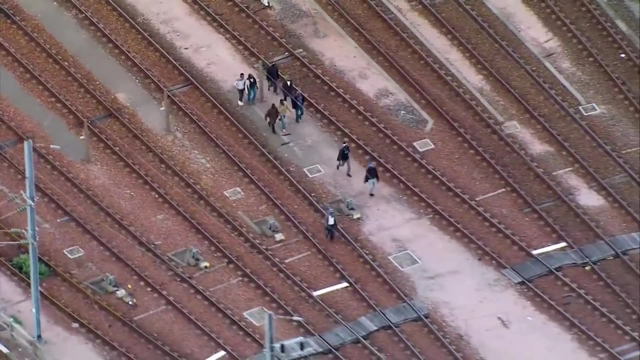 After battling fires and overcoming technical obstacles, the tunnel eventually opened. It proved to be a commercial success, moving millions of cars and passengers annually. despite the early setbacks, Even while it took longer than the stated 35 minutes, the trip time was still much shorter. 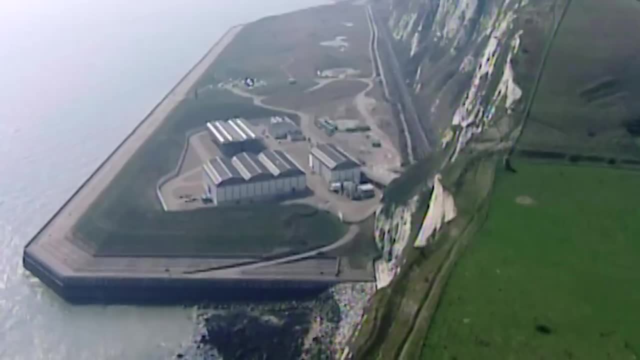 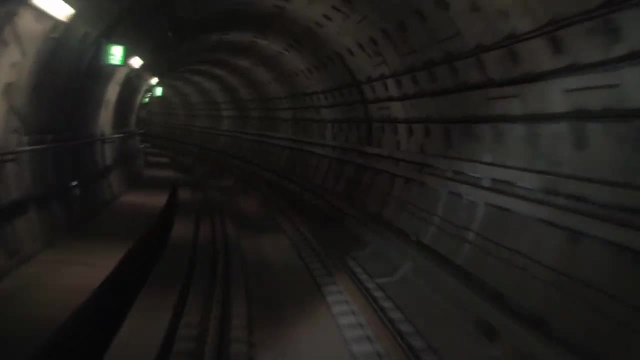 than that of ferry crossings. However, the Channel Tunnel's legacy remains complex. It stands as a testament to human ingenuity and the ability to overcome immense challenges, But it also serves as a cautionary tale about the pitfalls of ambitious projects. the risk, 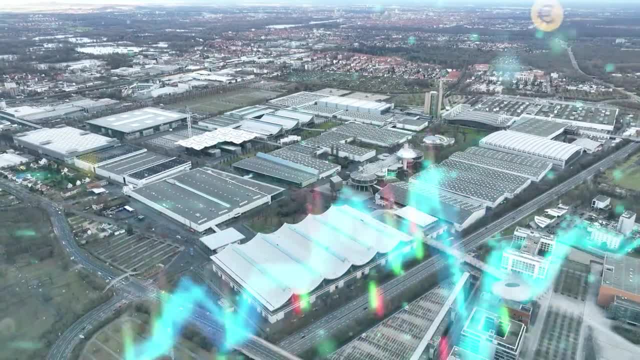 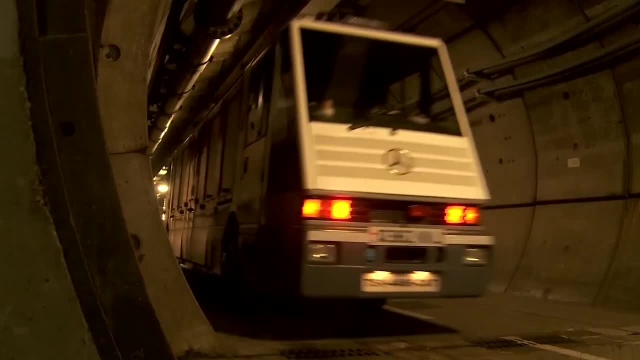 of underestimating technical difficulties and the financial burdens that can cripple even the most promising ventures. Even today, the Channel Tunnel, while a thriving transport link, carries the echoes of its turbulent birth, a reminder that the path to innovation is often paved with unexpected 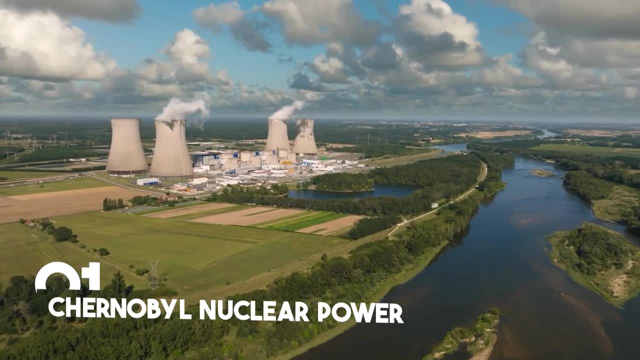 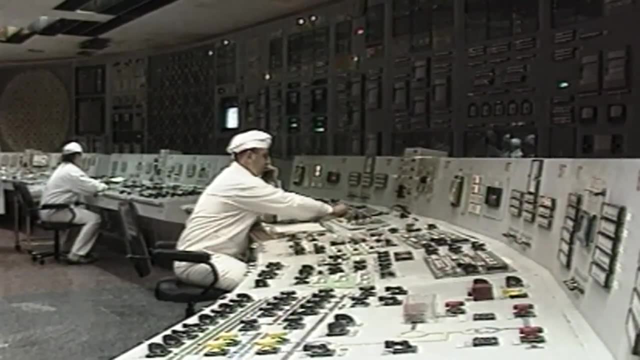 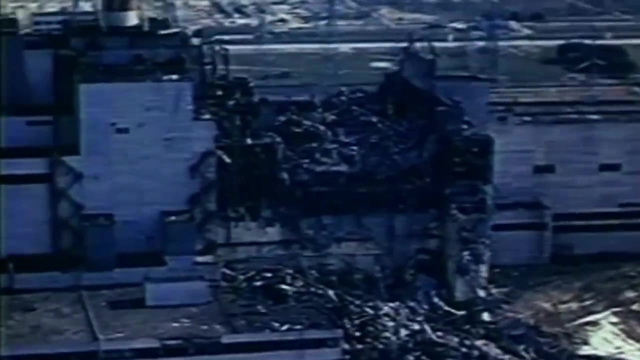 detours and financial potholes. Number 1. Chernobyl Nuclear Power Plant. On April 26, 1986, a seemingly routine safety test at the Chernobyl Nuclear Power Plant in Ukraine spiraled into a nightmare. Reactor 4 exploded, unleashing a radioactive cloud that choked the skies and blanketed. 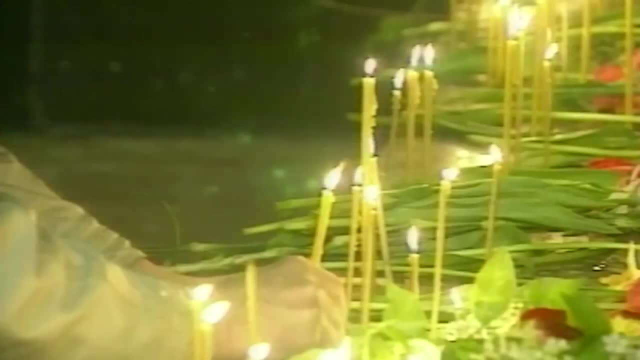 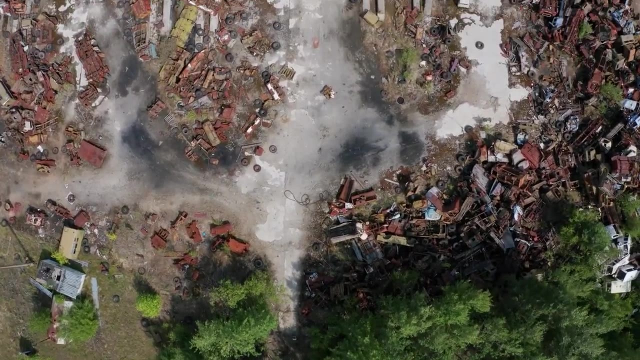 much of Europe. This wasn't just a technological failure. it was a human tragedy etched forever into history, a stark reminder of the devastating potential of nuclear energy gone wrong, The explosion spewed radioactivity. The nuclear power plant had radioactive material for ten days, contaminating vast swaths of 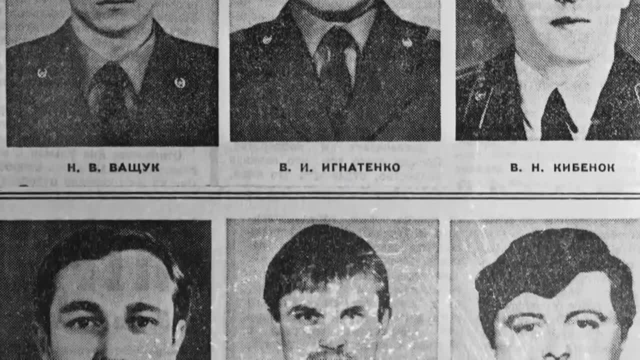 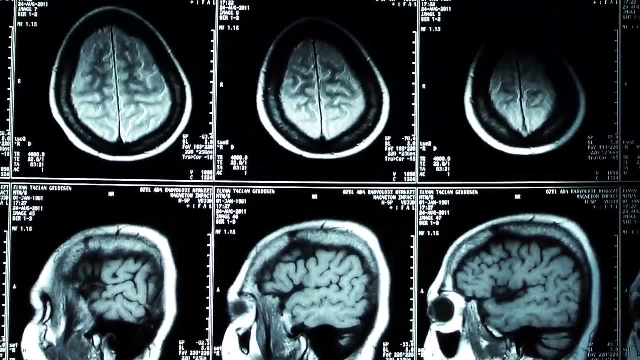 Ukraine, Belarus and Russia. While the immediate death toll was around 31,, thousands more succumbed to radiation exposure in the months and years that followed. The health consequences continue to this day, with an estimated 4,000 additional cancer deaths attributed to Chernobyl.